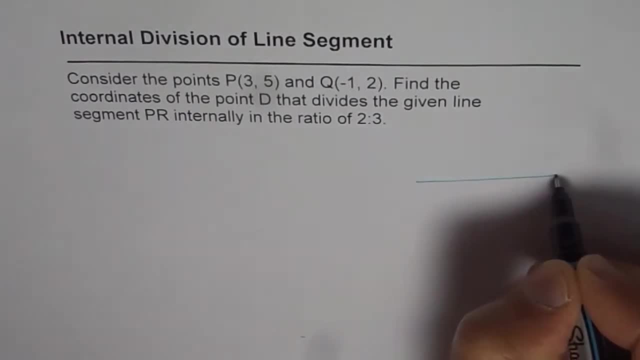 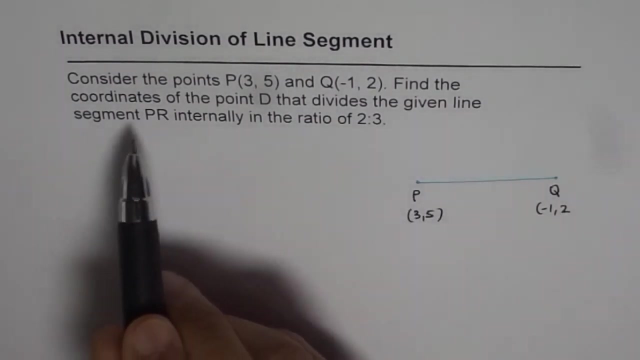 So what we are given here is, let's say that's the line segment right Where points P and Q are given to us. P is 3, 5 and Q is minus 1, 2. Find the coordinates of point D that divides the given line segment in the ratio of 2 is to 3.. 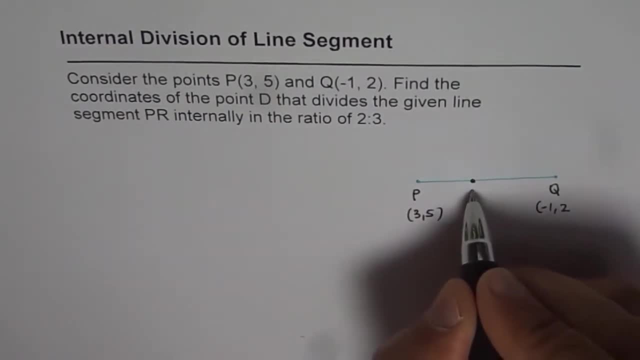 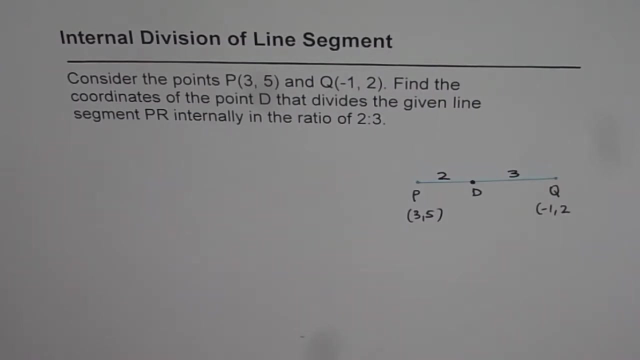 That means if D is somewhere here, so that we have this ratio. That means P to D is 2 and D to Q is 3, right? So for that we have derived a formula And in this particular example I am going to use the formula to get the answer right. 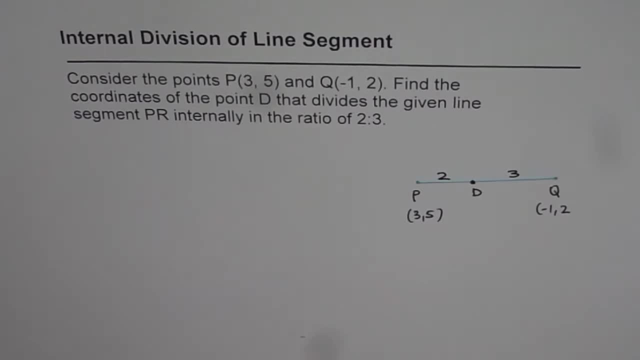 So how to derive the formula? You can look into my video on that, which is in the same playlist right Now. so to derive the formula, what we really do is we take an outside point O And then we join this point with. 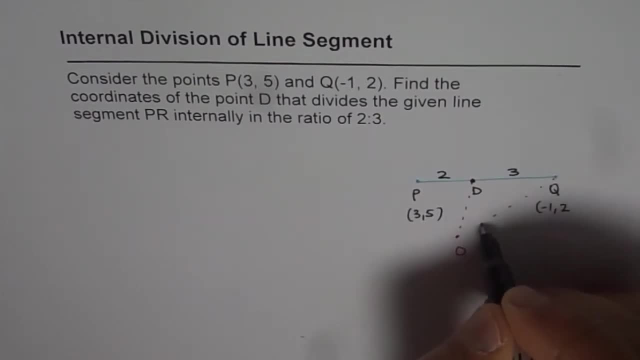 P and Q and D, So it kind of becomes a vector. Do you see that? From O, And that helps us to figure out the answer right. So O, if O is the origin, then it becomes a position vector, right? 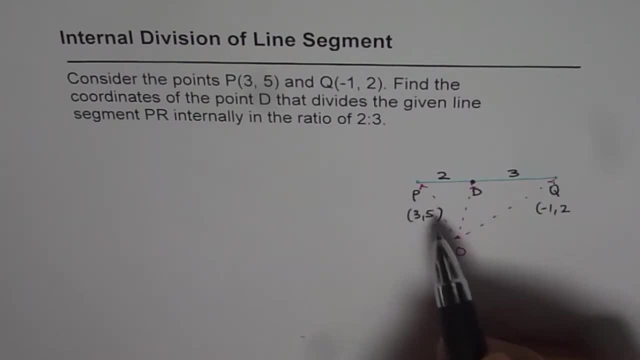 So if I write P then it becomes OP, right? So in this case, when I am writing the formula, I'll use the point external, point O, And so it becomes kind of familiar. Otherwise I could have used point P as a vector, P, which will represent the position vector. okay, 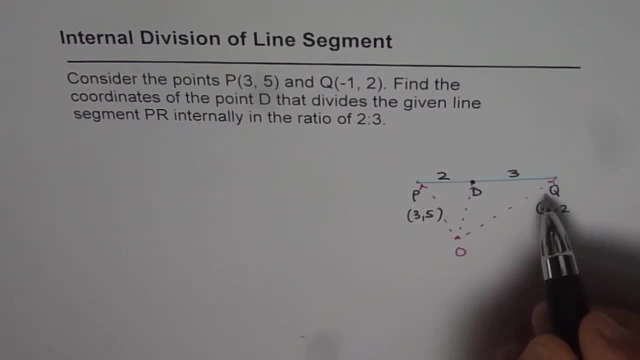 And OD as vector D and OQ as vector Q. So that could give me a position vector. So we can do that also right. But at present, since I have drawn this, let me write it in the terms of OD equals to the ratio is 2 is to 3.. 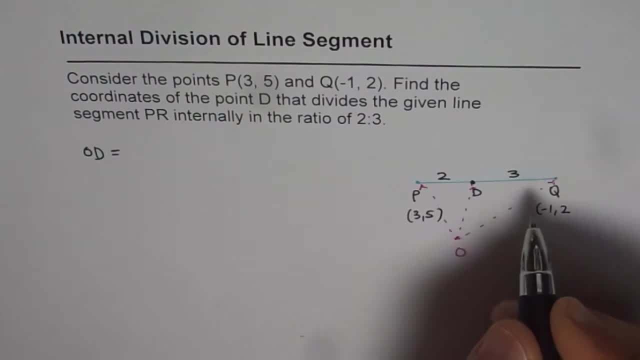 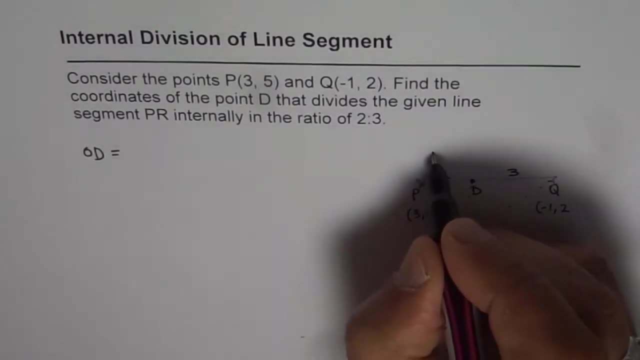 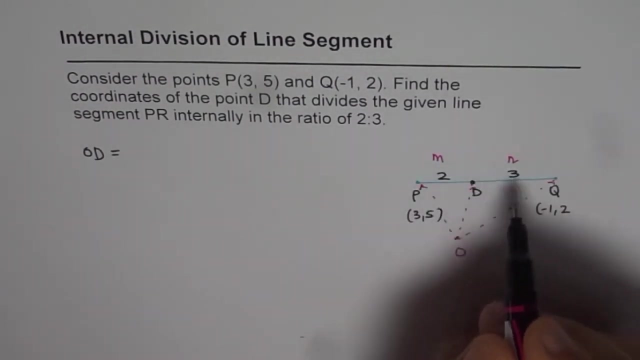 So it is 3.. Or let me write down the Formula first. First, if the ratio is, Let us say that the ratio is M is to N. Okay, If the ratio is M is to N, in that case the formula is N divided by M plus N times OP. 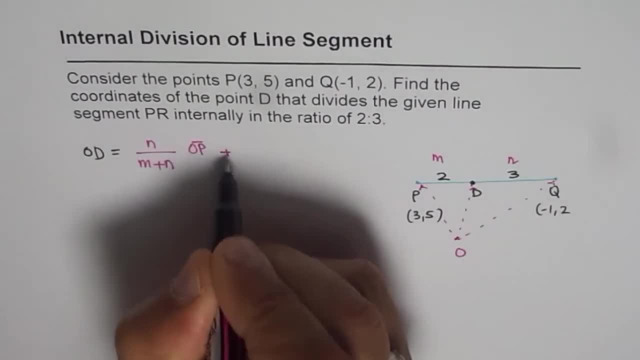 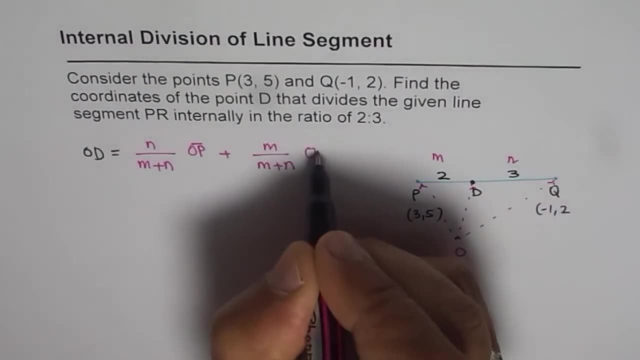 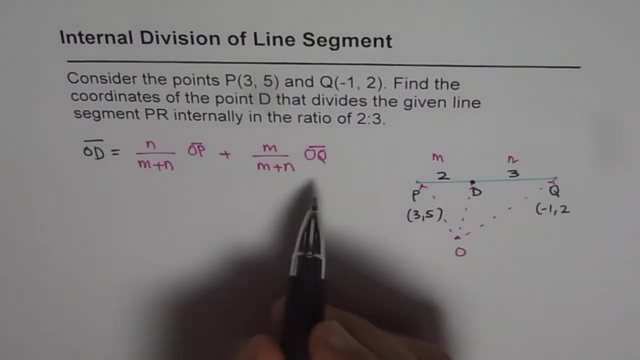 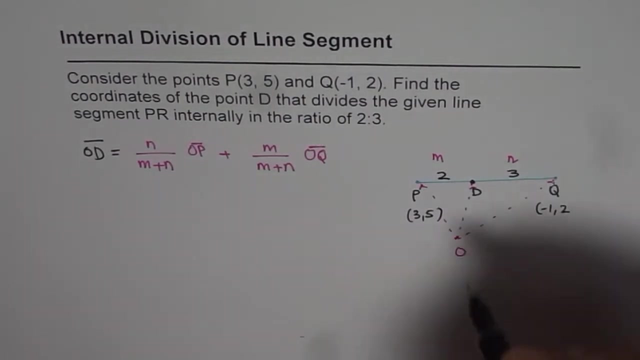 plus M, divided by M plus N times OQ, Right. So that is the formula right, Which let me write down as a vector itself. So OD, basically, is a vector D, let us say. Let me write down these vectors here. 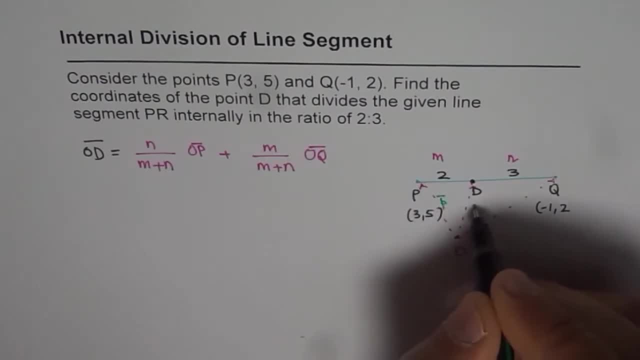 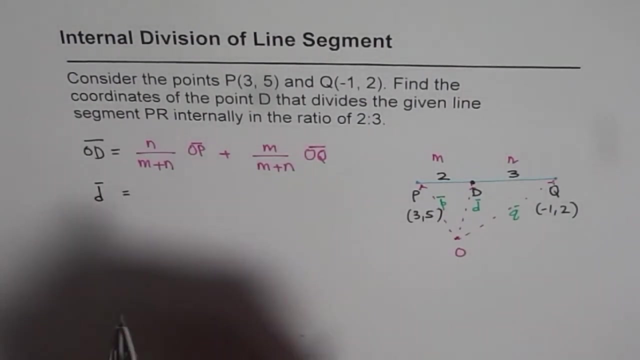 So let's say we are talking about vector P here, which is a position vector, D is a position vector And Q position vector for Q right. So in terms of these position vectors, I could write this as: D equals to N is 3, right. 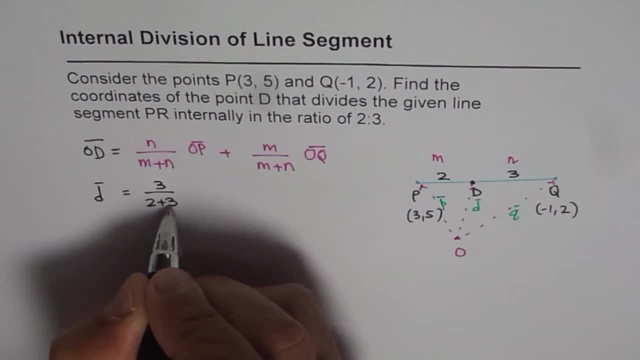 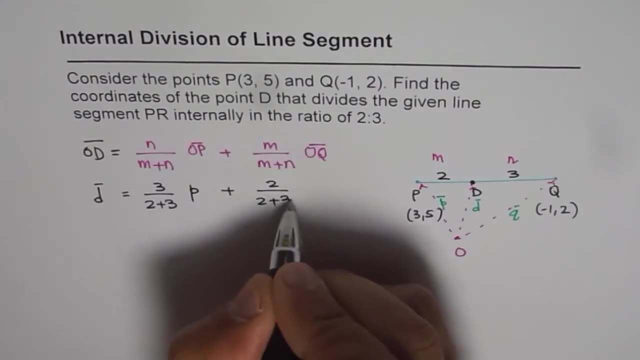 So it is 3 over 2 plus 3.. OP is position vector P plus 2 over 2 plus 3.. OQ is position vector Q. Okay, Now the point represents a position vector. So we get: D is equals to 3 over 5 of point P, which is 3.. 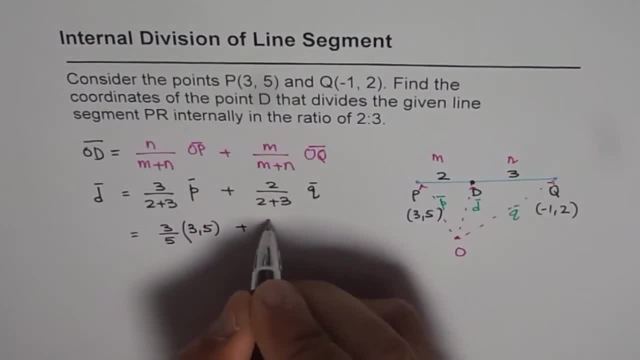 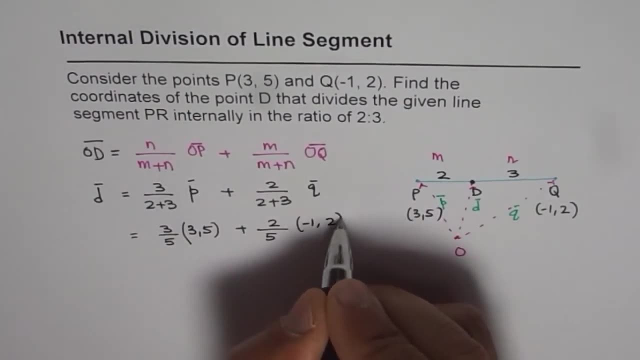 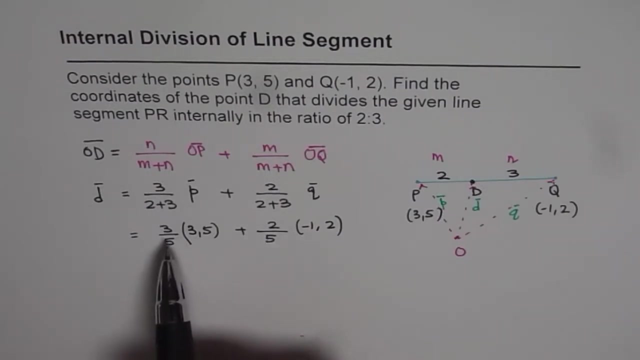 So we get: D is equals to 3 over 5, plus 2 over 5. And Q is minus 1, 2.. You'll also notice that, since they are collinear points, if I add these two coefficients I'll get 1.. 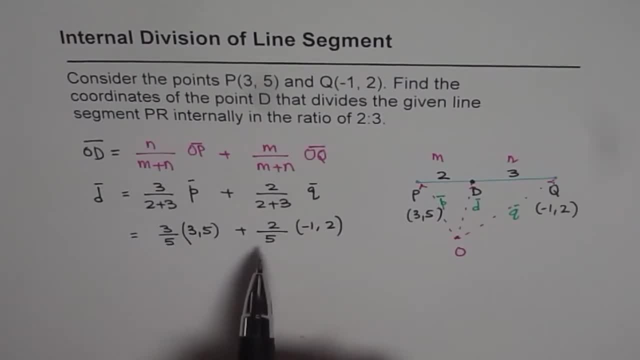 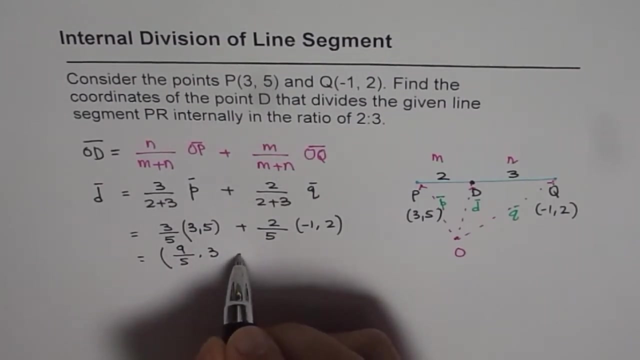 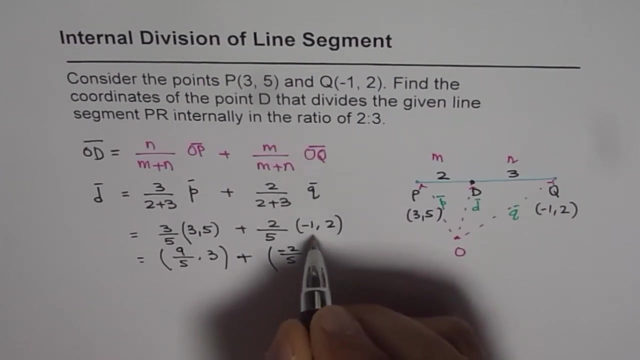 3 plus 2 is 5.. 5 over 5 is 1.. So there is another important point to notice here. okay, Now let's solve for the coordinates of D, right, be 9 over 5, and this is 3, and the coordinates let me write plus minus 2 over 5, and here: 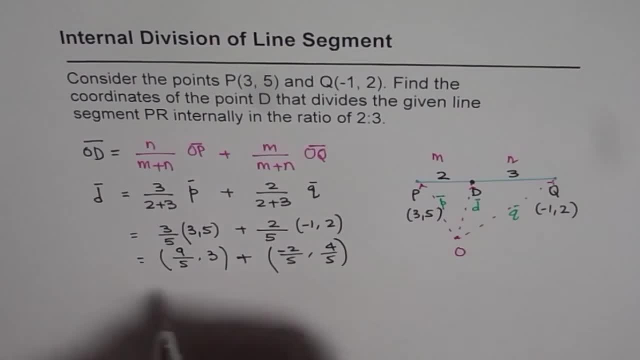 we get 4 over 5.. So that gives me the coordinates for D. we just add 9 and this, which is 7 over 5, and 3, so it's 15 plus 4, which is 19 over 5.. So these are the coordinates for D. So